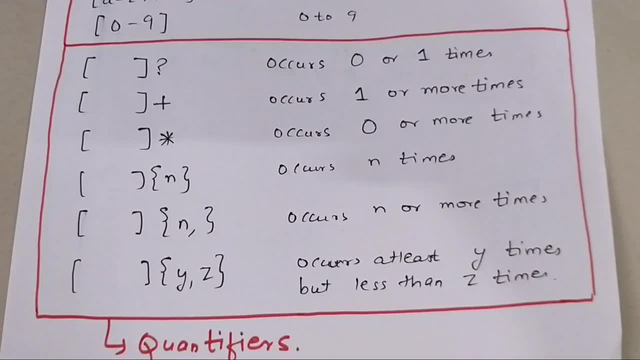 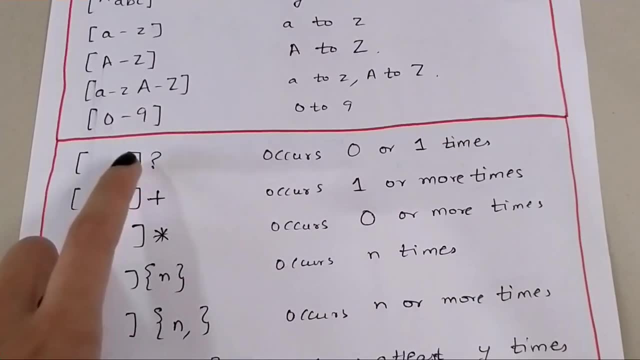 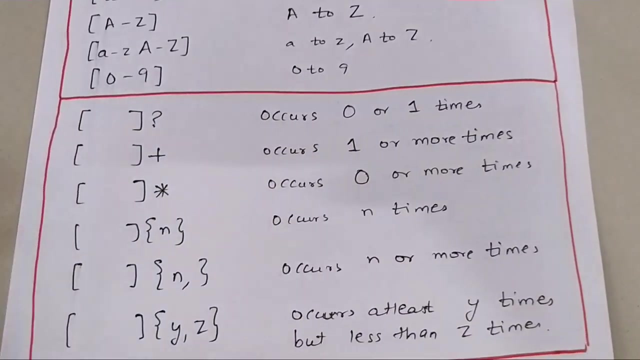 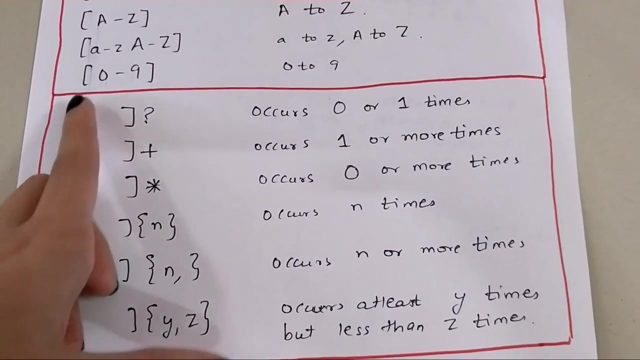 these are quantifiers. Let's understand what are quantifiers in brackets? Okay, So, basically the same bracket and whatever. you can write anything, any of this inside this, but but using quantifiers we can. we can tell the computer about the repetition. Okay, So when we write question mark, it basically means whatever is written inside this. whatever the rule is there, it can occur zero or one times. Okay, There's a question mark. 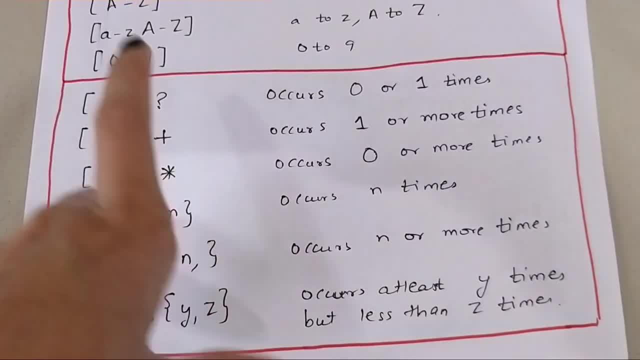 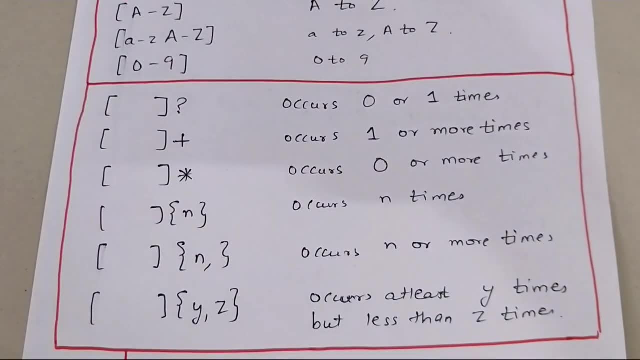 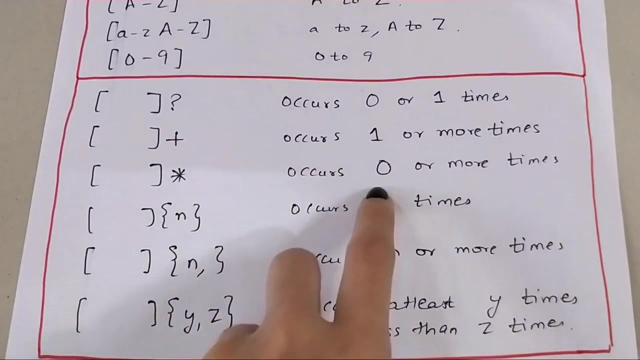 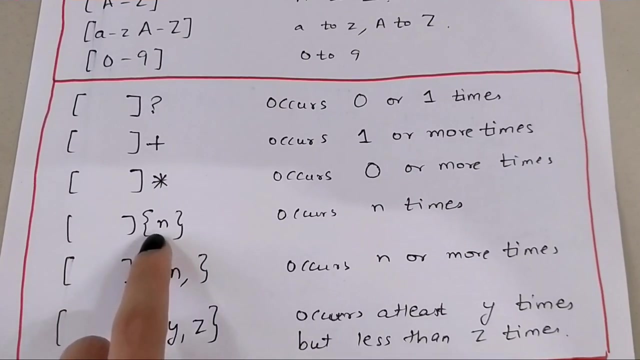 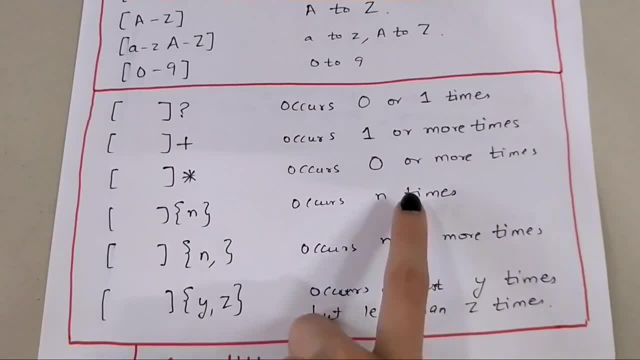 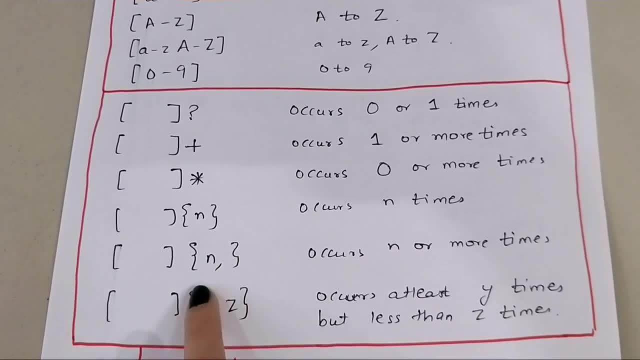 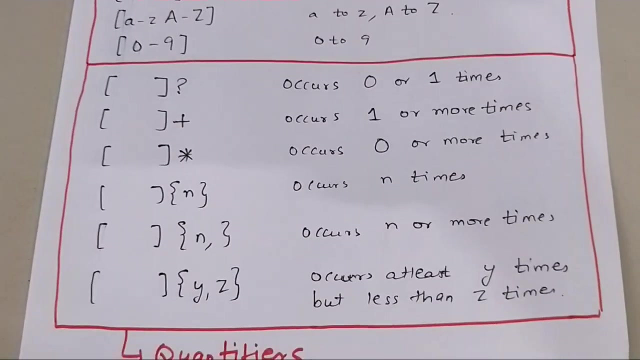 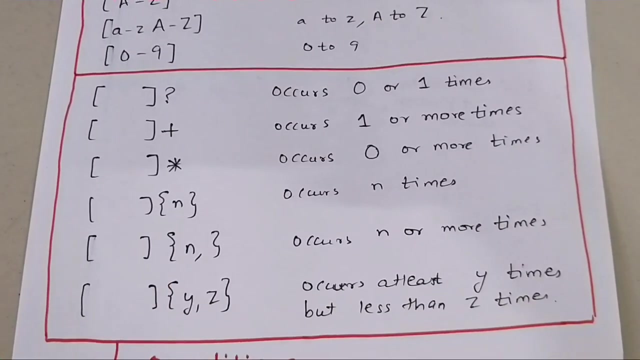 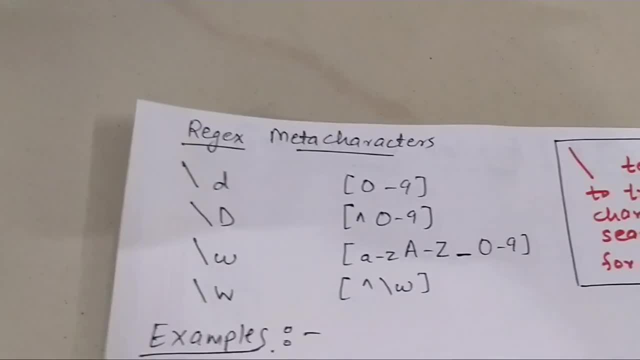 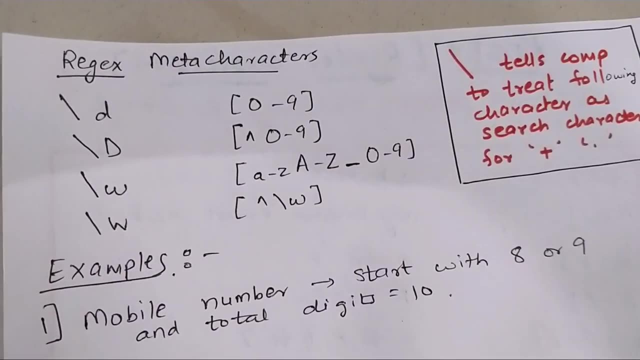 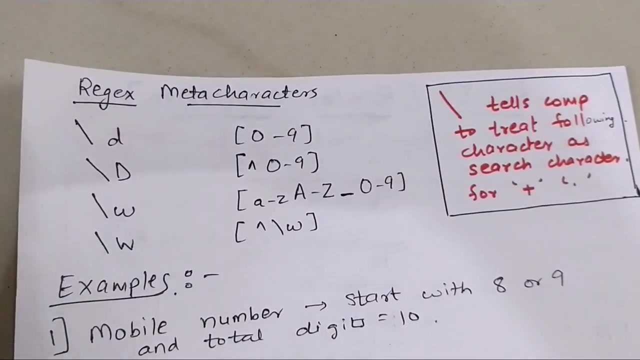 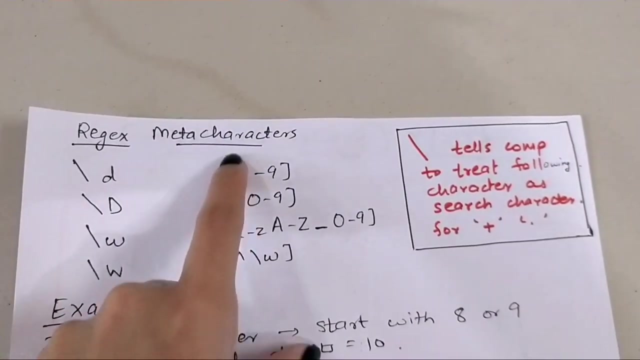 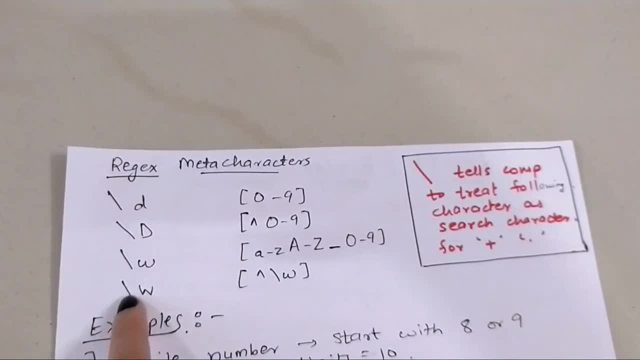 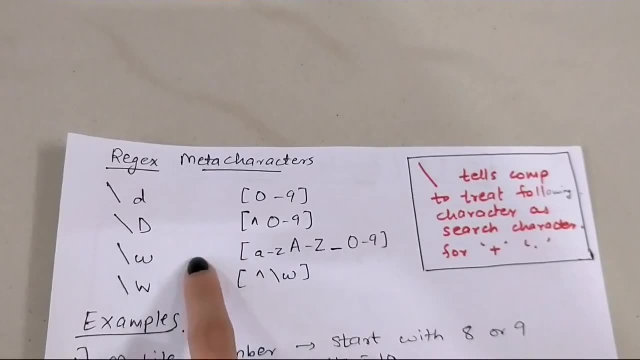 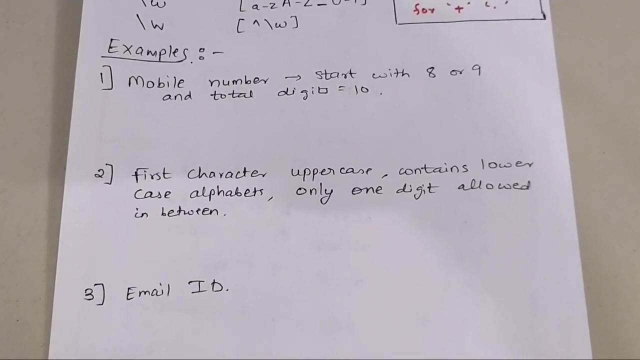 small a to z, capital a to z, 0 to 9, all of this, and when you write this is capital w. i'm sorry it doesn't look like capital w, but this means it is a negation of the above. okay, now let's see three examples, and after that i am sure that your confusion will go away, if there is. 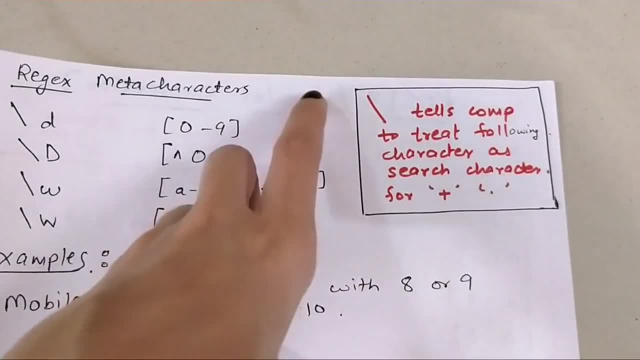 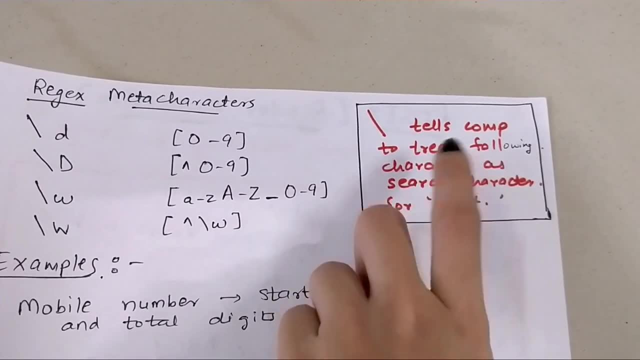 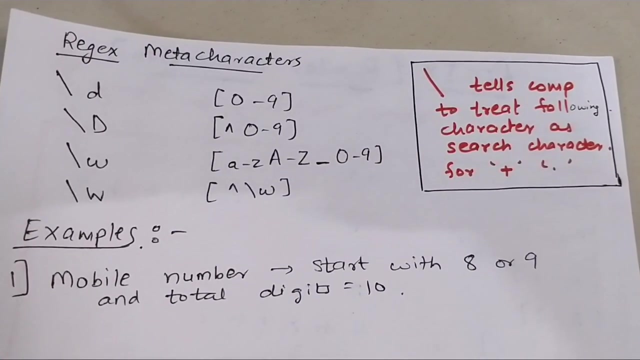 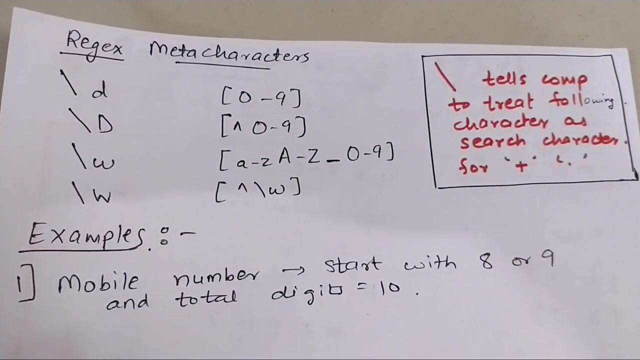 okay, and before that let me tell you what this uh backward slash means. okay, now, backward slash will tell computer, computer to treat the following character as search character. now, for example, if you want to search in your- um, you know- regex expression, if you want to actually search the plus sign or the dot sign or the backslash itself, you cannot simply write it. 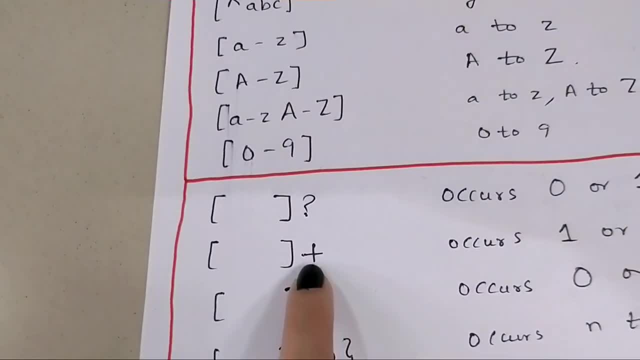 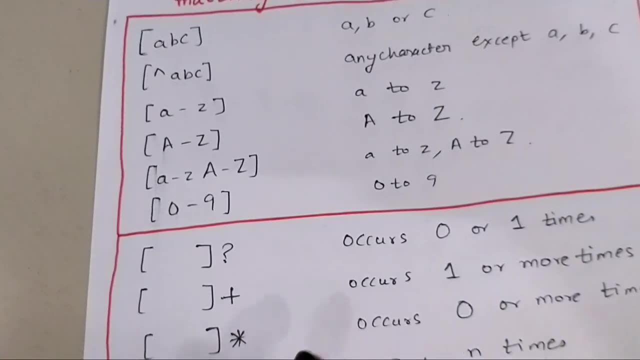 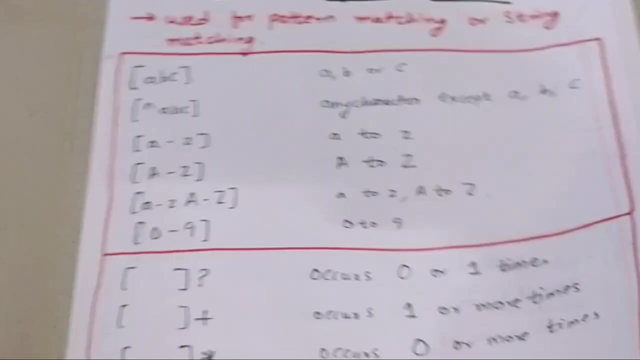 because it means something else, because plus sign also means something over here, the, the, the hyphen means something else over here. so if you want to search hyphen, okay. hyphen itself, okay, because we cannot write hyphen just like that. okay, if you want to want the computer, 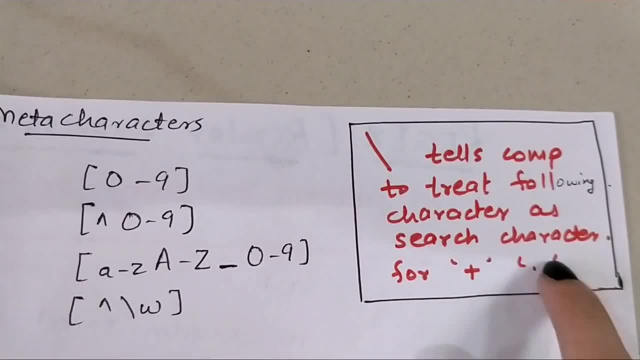 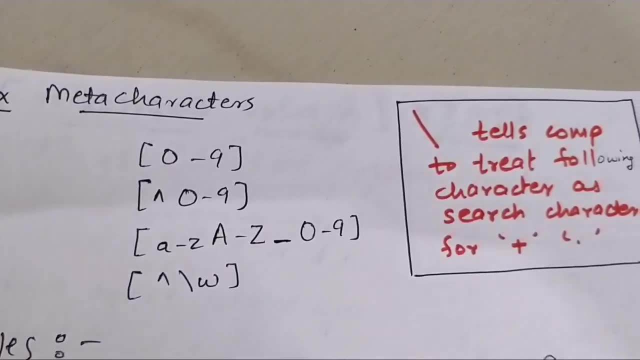 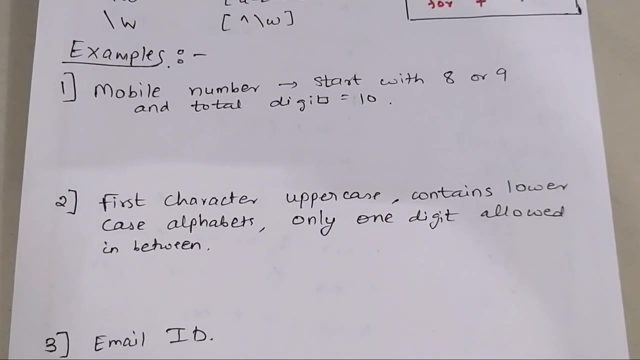 to actually search, uh, the high search hyphen, or plus sign or dot, you have to write this, this backslash, before it. so this is known as the escape character. so you will understand this better in the email id example. okay, so let's see the examples. so the first example is it should check. 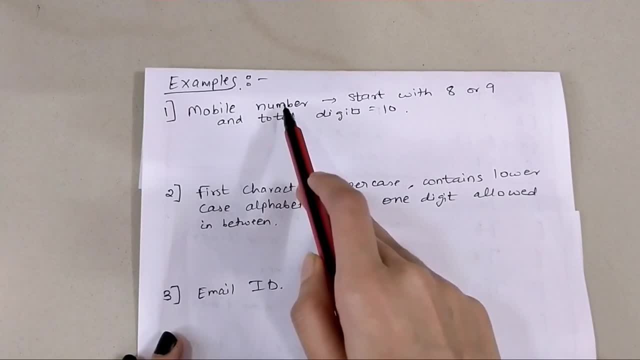 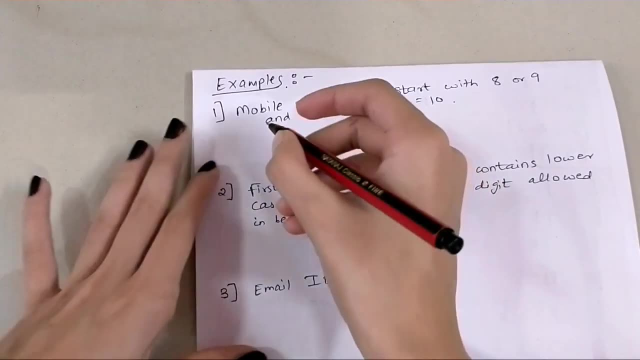 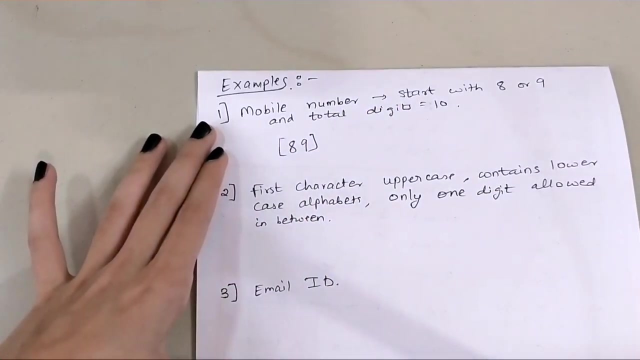 if it is a mobile number, okay. okay, the pattern should check if it's a mobile number. so it should start with either eight or nine and the total number of digits should be ten. so what i'm going to write is okay. so the first digit can be either eight or nine. okay, so basically, it will uh take. 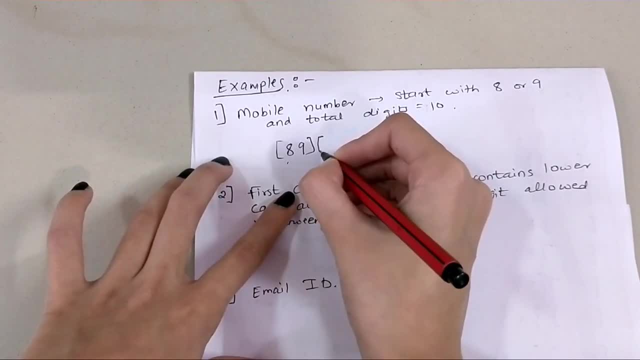 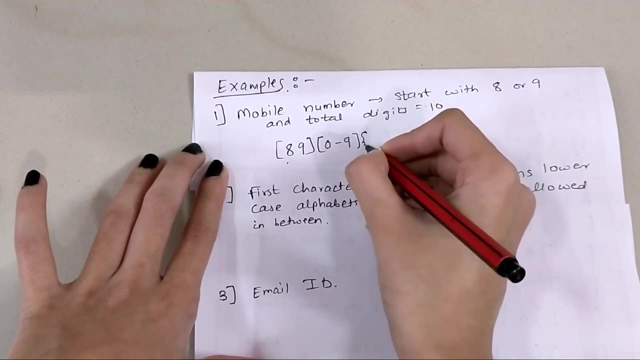 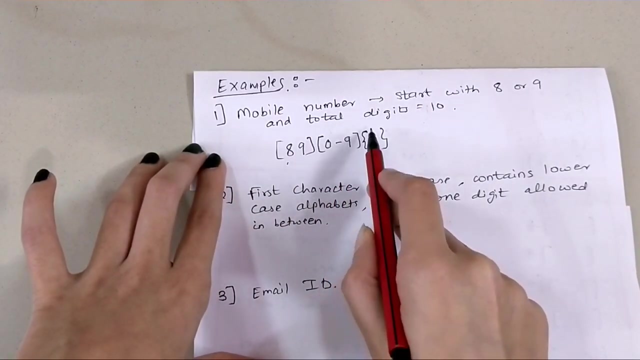 anything, uh, either eight or nine, okay, and any digit that can. there can be any digit in between, so zero to nine, and this has to be nine, so zero to nine, it has to uh collect uh any digit from zero to nine. how many times? nine times? okay. so when i write uh nine in brackets, 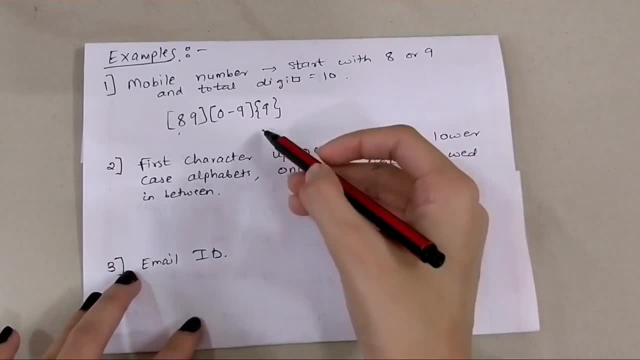 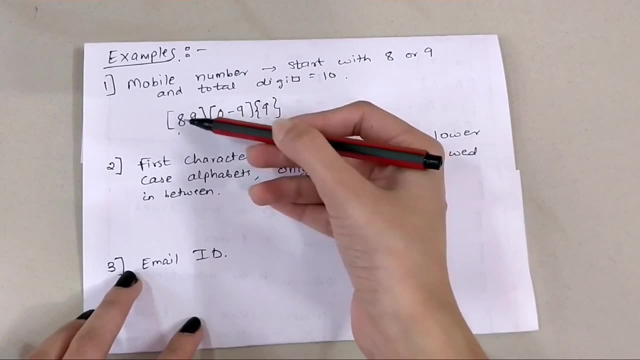 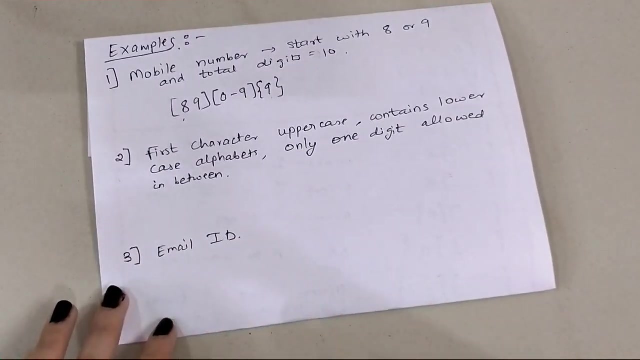 uh, it means it has to repeat nine number of times. why nine? because i will take one digit from here, so it will be either eight or nine and total should be equal to ten. so this is how i will, how i will check if it is a mobile number or not. now, second example is the first character. 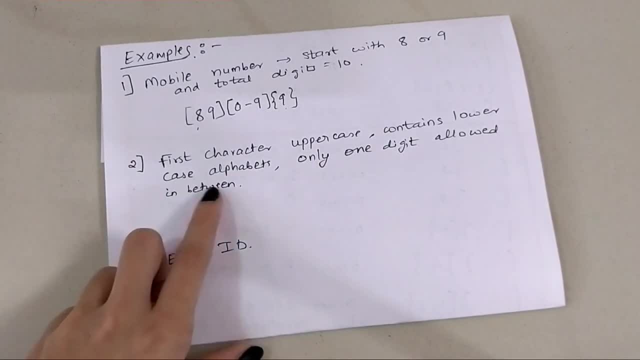 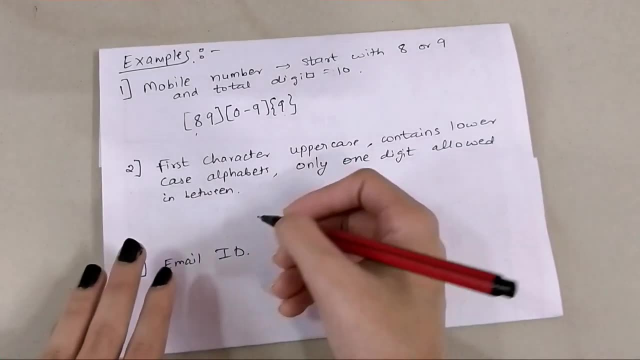 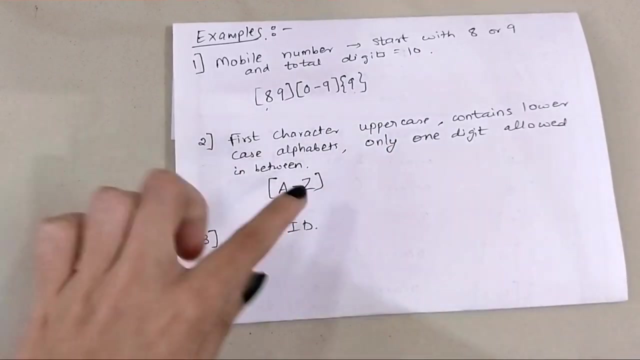 uh should be uppercase and it should contain lower case alphabets. okay, and there should only be one digit, uh, in between them. okay, so the first digit has to be an uppercase. so i will write a to capital z, so the for uh anything, any uh, anything from a to z will be collected one. 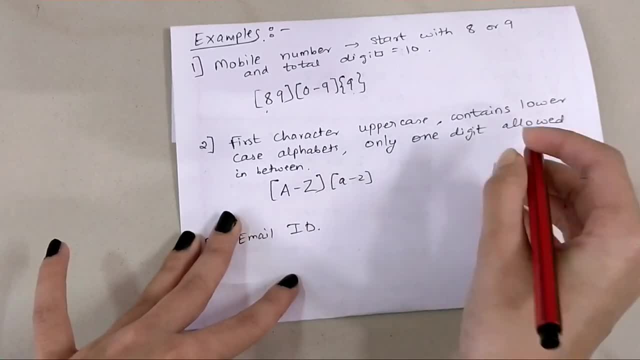 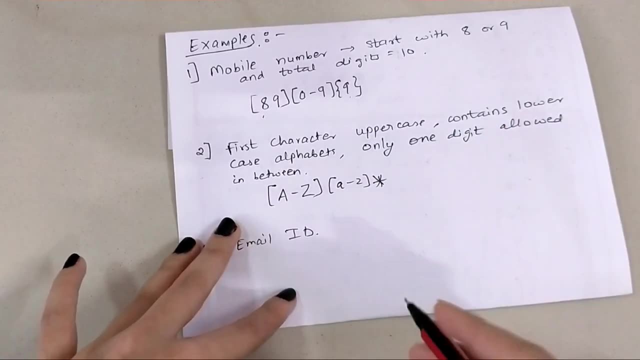 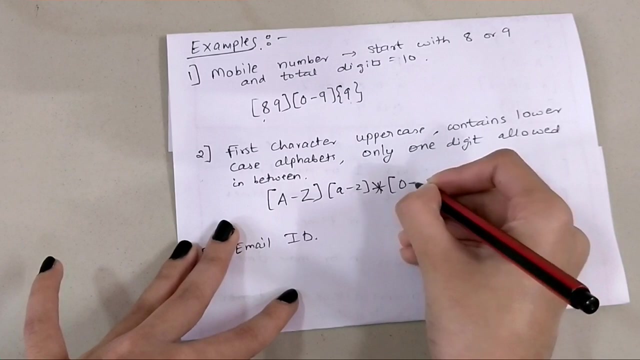 then small a to z, because i have said it should contain lowercase alphabets. okay and uh. these can repeat how many times. asterisk means zero or n number of times, and there has to be only one digit in between them, zero to nine. so i'm not going to write. 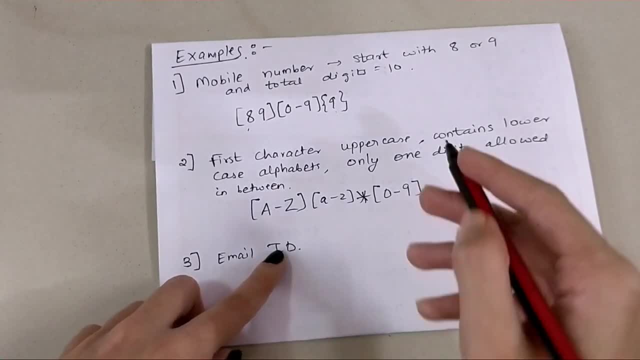 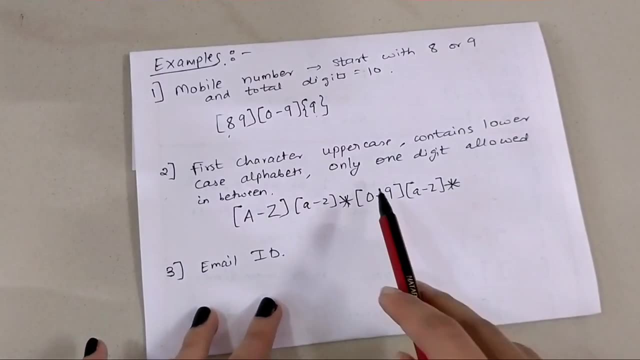 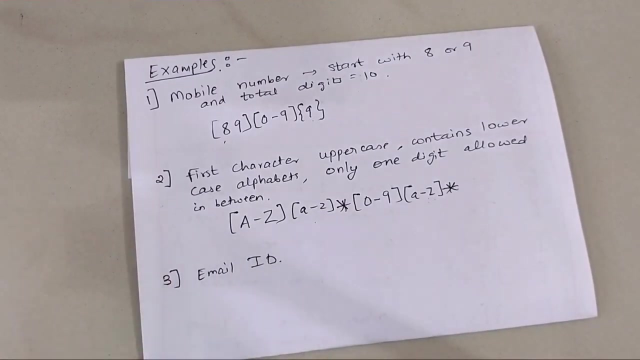 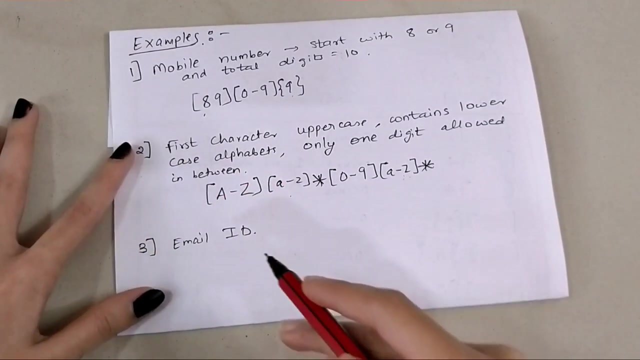 anything, because it will take only one out of it. okay, and then again i will write a to z and then a strip. so basically, there will be one digit allowed between the lower cases and there will be one uppercase um ahead of this. okay, okay. so this is the second example. now third example is of an email id. 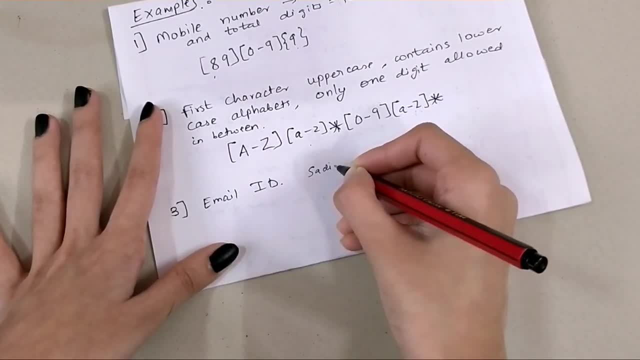 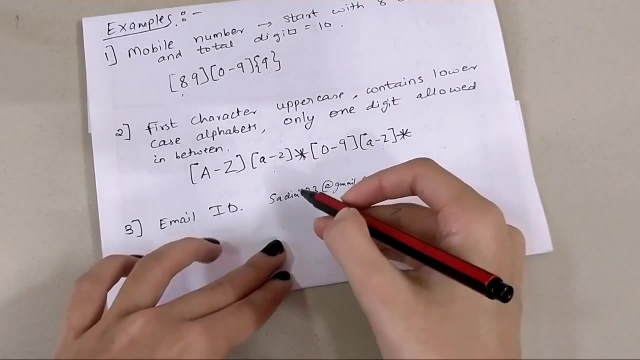 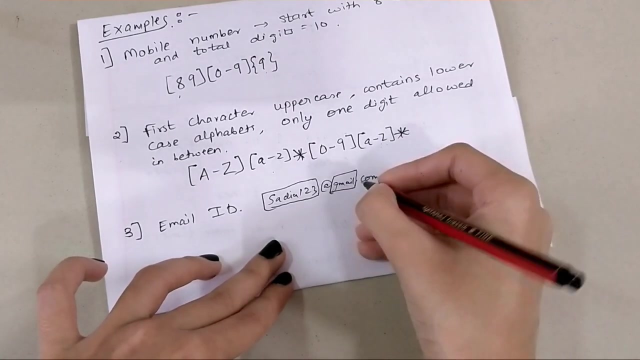 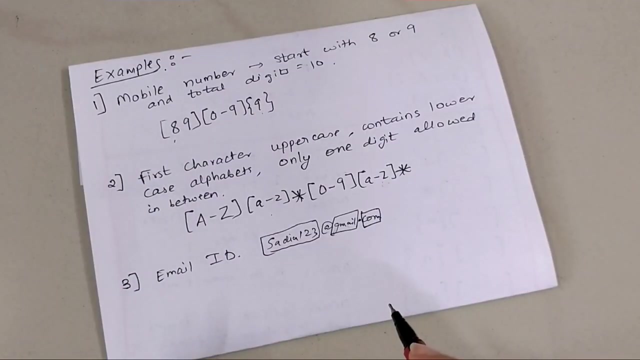 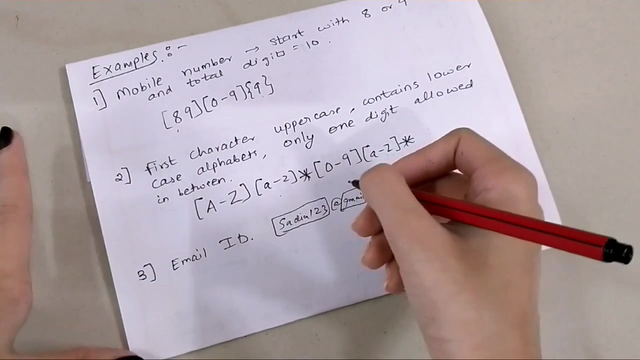 now email id can be something like sadia, so email id is going to be something like sadia123.gmailcom. so i want to allow this. so there are going to be like three parts to it. okay, now, the first part is sadia123. okay, now i want to allow this first part to have alphabets, uppercase, lowercase and digits also. 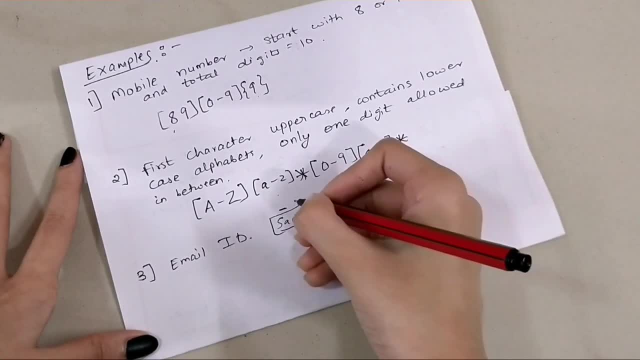 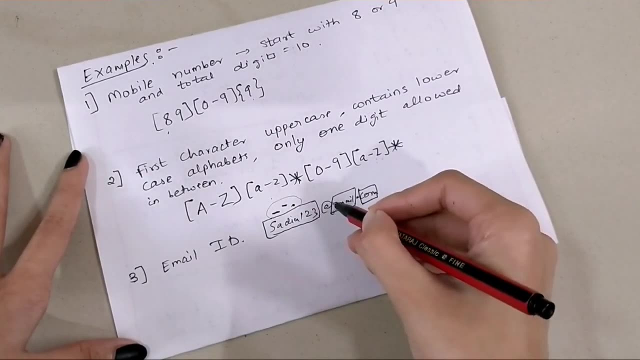 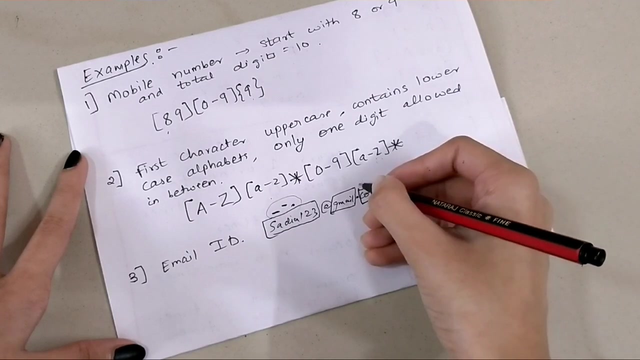 and at the same time i also wanted to have underscore hyphen: full stop. i want these letters to also be allowed in this. then i want an at okay. then i want some small uh lowercase alphabets over here. then i want a full stop over here, and then i want uh again. i want small letters. 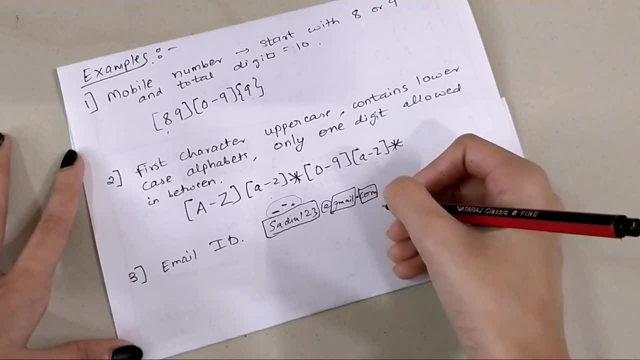 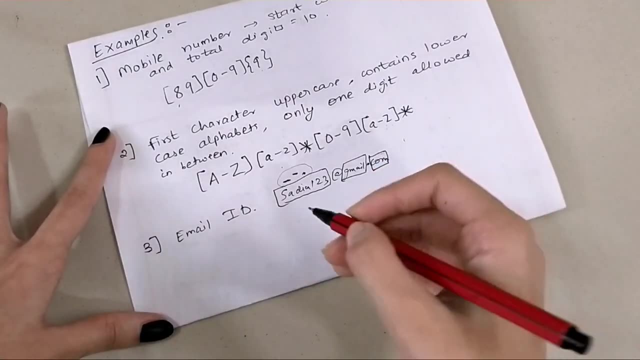 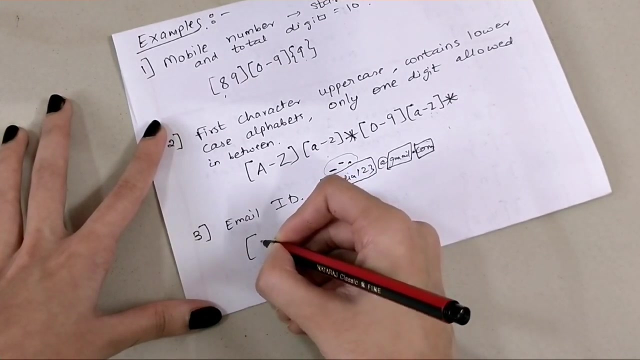 over here. it can either be dot com or dot in. right, it can either be dot com or dot in. it cannot be more than that, okay. so this is the example. let's try, let's try, let's do the first part, which is this box. so, um, i am going to allow small a to small, okay, a small z capital a to capital z. 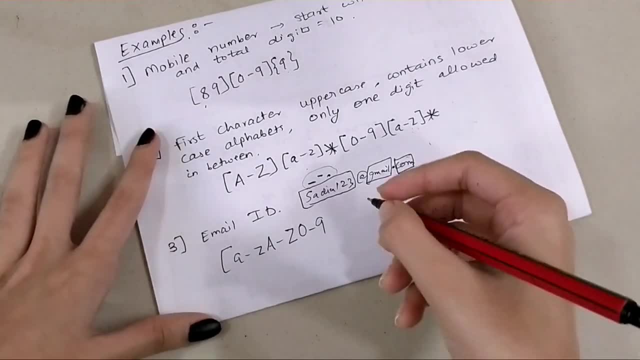 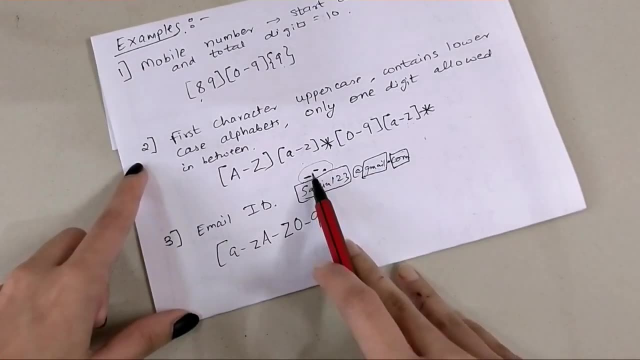 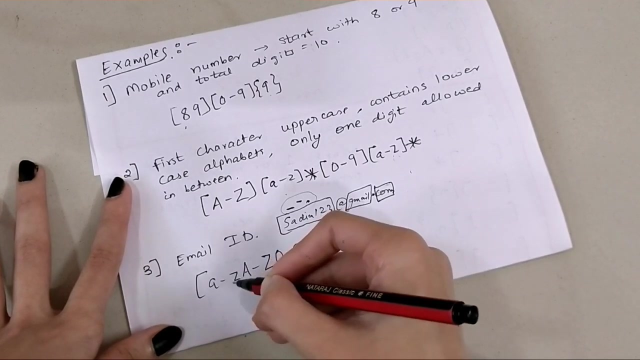 zero to nine. okay, so i'm gonna. so i allowed all this. then i want to allow underscore. okay, now i also want to allow hyphen. but i cannot allow hyphen, because hyphen has some predefined meaning attached to it, because a, a hyphen z is written. all of this already already written, but i 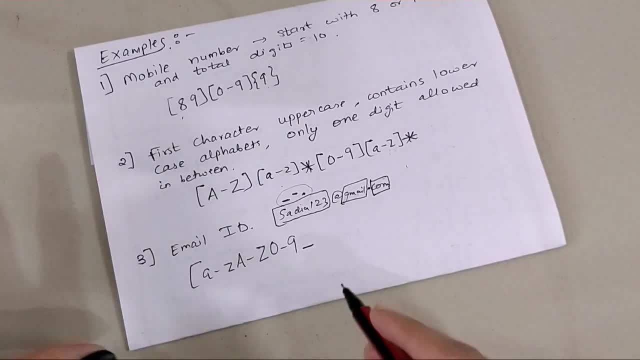 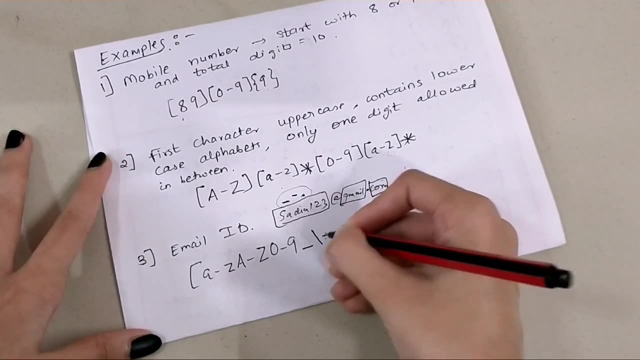 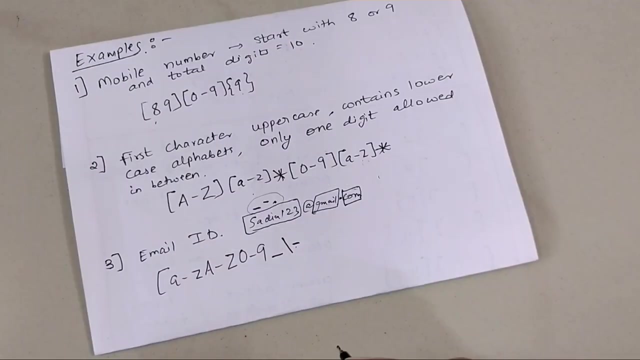 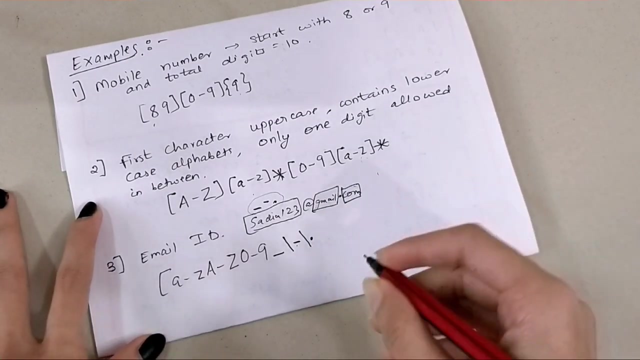 want it to be, uh, to be in the pattern, okay, so i will use escape, as i already explained. so this will tell the computer to take the second, uh, the next thing, um, as literal. okay, and then i also want it to select full stop. so i will write the escape: uh, escape. 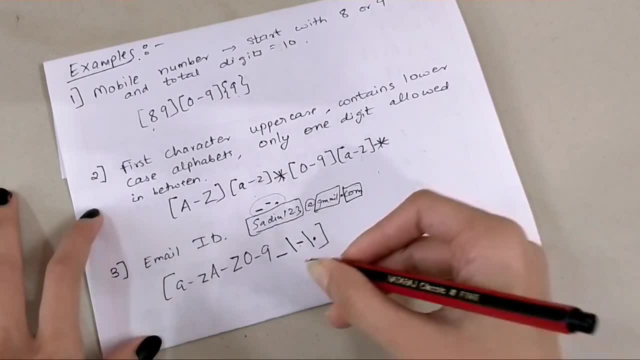 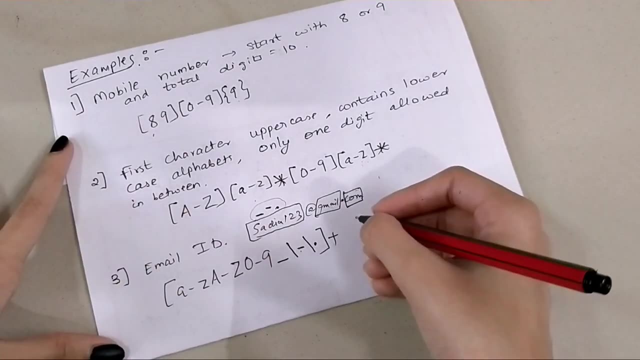 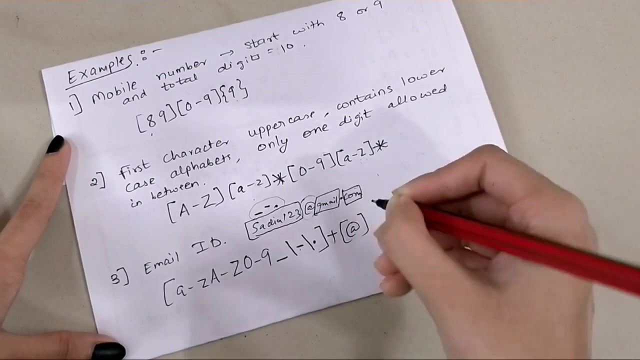 thing, and then the full stop, and then i will close it. i want this to repeat: repeat, okay- at least one or more number of times. okay, then i want add symbol, so i will write add, okay, if you do not write it in the square braces, it's still fine in this case, but uh, i 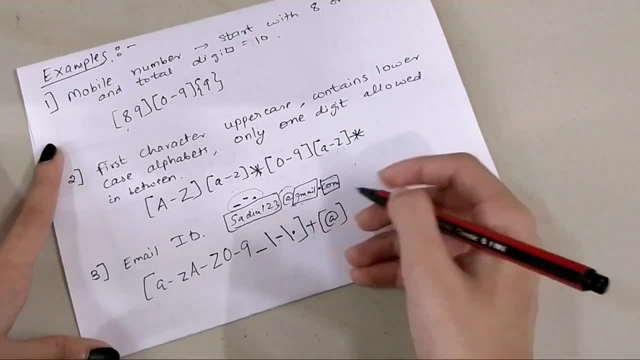 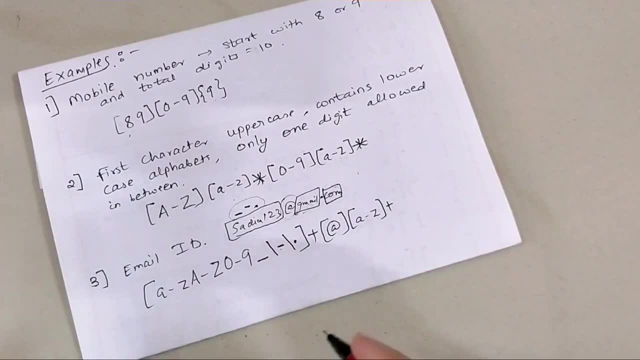 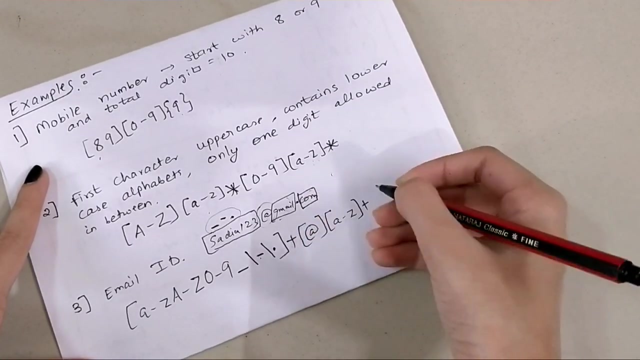 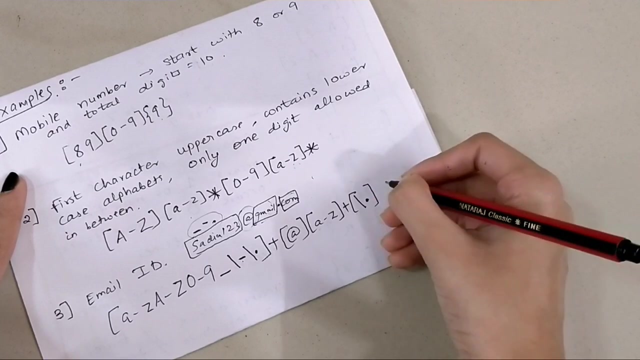 prefer writing. then again small characters over here. okay, a 2 small characters or ok, okay, which can repeat at least one times, and then okay, so till Gmail is done. now I want a full stop, so then I will take the skip thing full stop and then again. 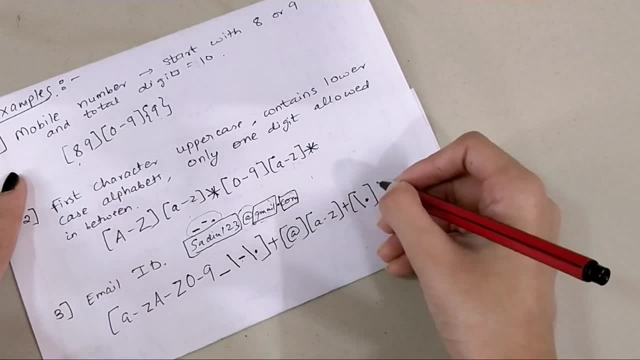 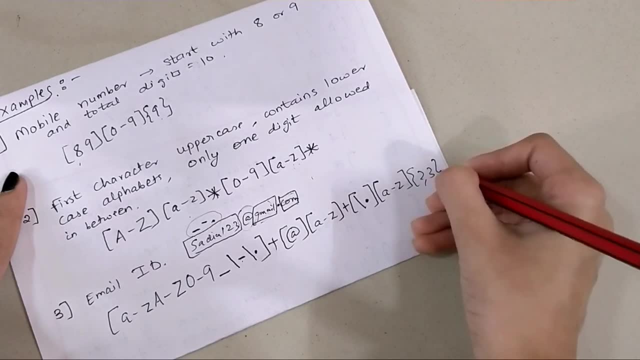 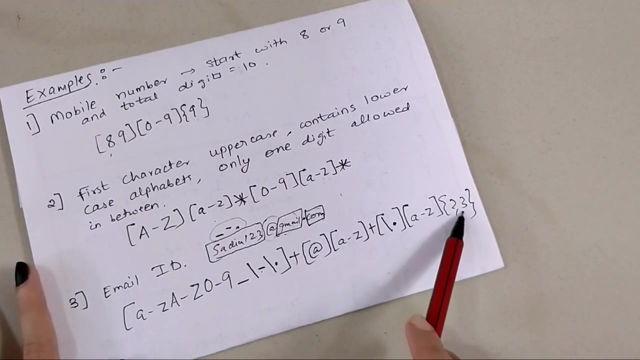 after that I need comcom or in so small, a to z, and this can repeat how many times. two to three. why two to three? basically it should at least have two characters, so at least dot in and not more than three because dot com. so basically two to three. two to three characters can be in this position. so I